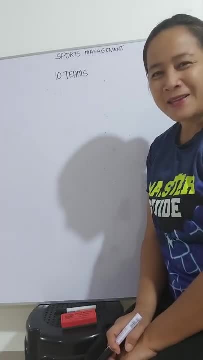 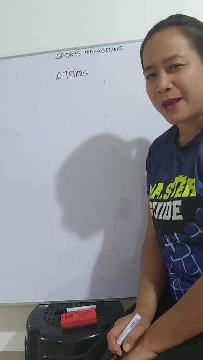 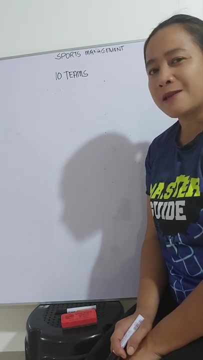 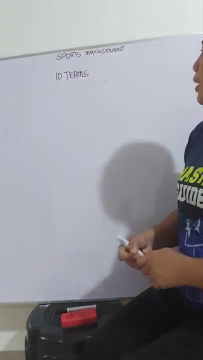 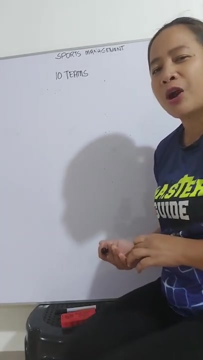 Good evening. Our problem tonight is 10 teams, So we'll be using single elimination under sports management. So when we say single, that is a knockout system. Once the competitor loses its chance, then the competitor will be eliminated right away, And so we'll be having the formula, which is n minus 1.. n represents to the number of teams, competitors and players. And minus 1 is constant, And so n is 10 minus 1.. The answer is 9 games, So there will be 9 games for the whole duration of the competition. Now let's proceed to power of 2 minus 1 to identify the number of buys. 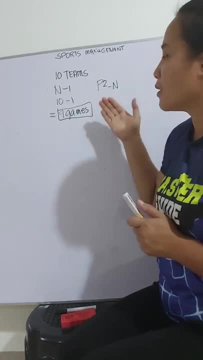 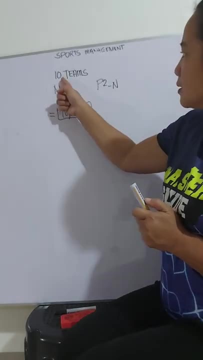 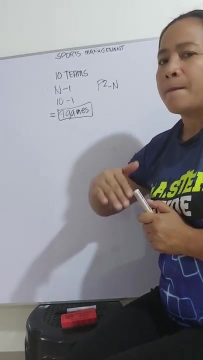 As you can see, power of 2 here is 16.. So why not 8?? Because the result is negative. Remember, Remember that it should be equal to the number of power of 2, or beyond to the number of our number of teams. 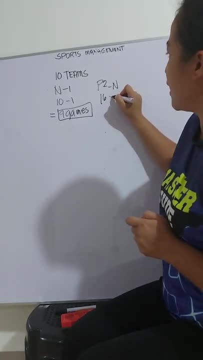 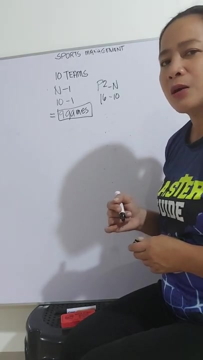 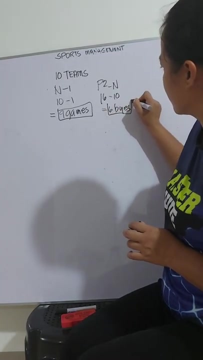 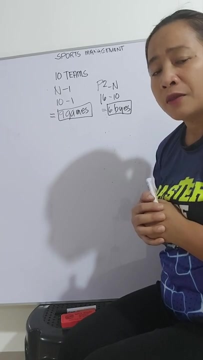 So we'll be using 16 minus 10.. After which we will subtract 16 minus 10.. So we have 6 buys Again, those who will be buys. meaning to say they're not the winners. So meaning to say they'll be moved to the next round. 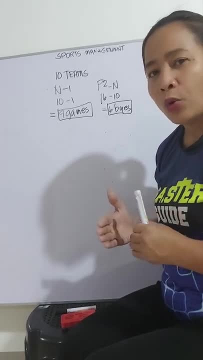 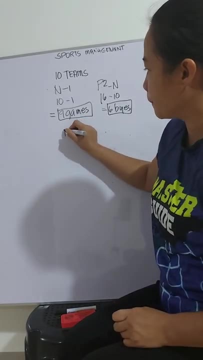 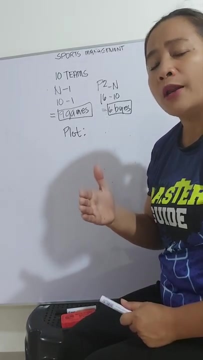 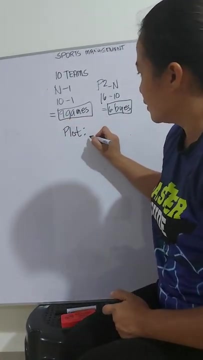 Remember, buy is just an advance or waiting. team players or competitors. Let's have the plot. This is to identify Who will be the game 1, the winner 1, game 2, until game 9.. And then don't forget to seed the tournament. 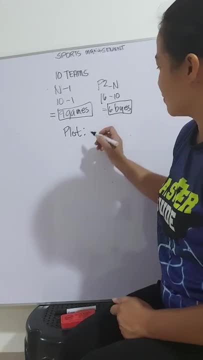 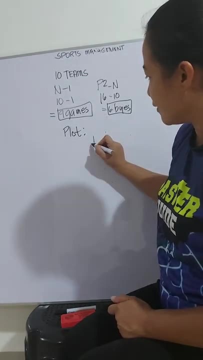 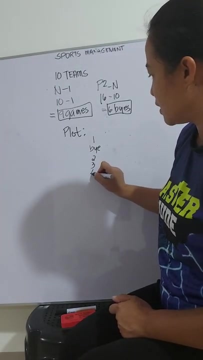 So when we say seed, that is to avoid mismatch, Supposing team 1 is one of those best teams, So we will put: buy here, Team 2, not And team 3? Team 4, one of those 5.. Buy 6., 7., 8. Buy 9. Buy 10., 11., 11., 12., 13., 14., 15., 16., 17., 18. 19.. 20., 21., 22., 22., 23., 24., 25., 26., 27., 28., 29., 30., 31., 32., 33., 33., 34.. 34., 35., 35., 36., 36., 36., 37., 37., 38., 38., 39., 40., 41., 42., 42., 43., 43.. 44., 44., 45., 46., 46., 47., 48., 49., 49., 50., 51., 52., 52., 53., 53., 54., 55.. 56., 57., 58., 59., 60., 61., 62., 63., 64., 65., 66., 67., 68., 69., 69., 70., 71.. 72., 72., 73., 74., 75., 76., 77., 78., 79., 80., 80., 81., 82., 83., 84., 85., 86.. 87., 88., 89., 90., 91., 92., 92., 93., 93., 94., 94., 95., 96., 97., 98., 99., 100.. 100., 100., 100., 100., 100., 100., 95., 95., 90., 101., 102., 103., 104., 103., 104., 105., 105.. 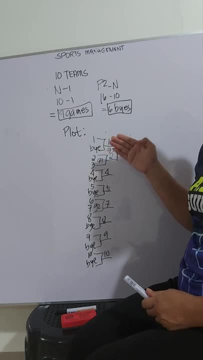 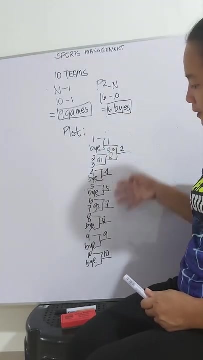 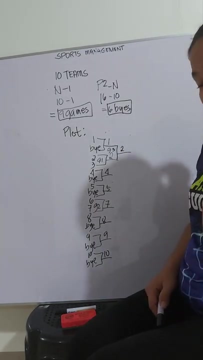 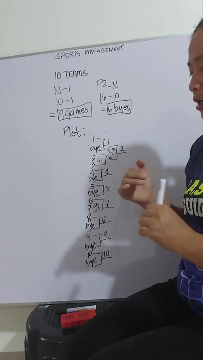 106., 107., 108., 109.. although, with this situation, you can create or you can let others to play first, but let's make sure that we have this in order, okay, although you can reshuffle or you can exchange those who will. 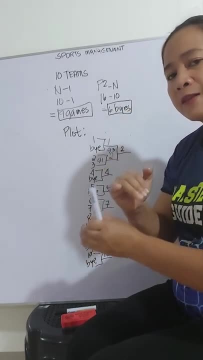 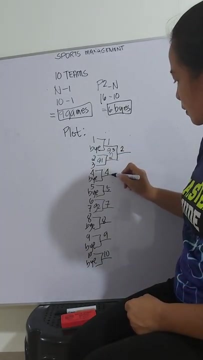 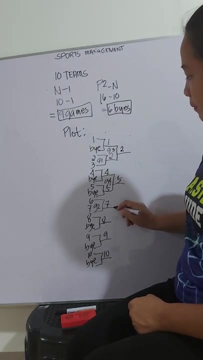 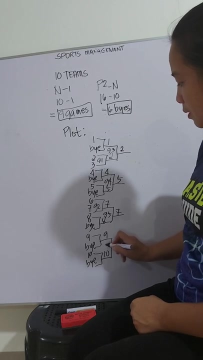 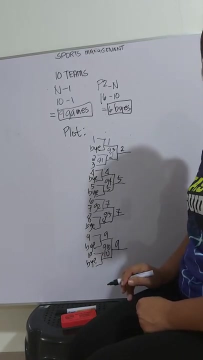 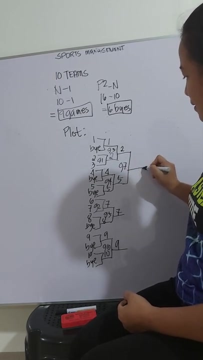 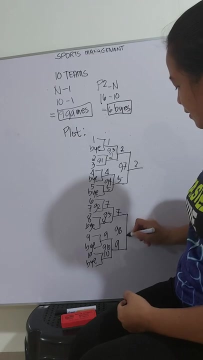 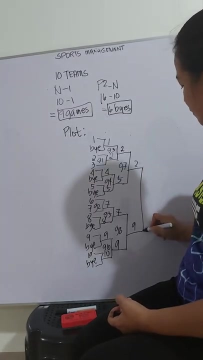 be the next or who will play in the next game. it's up to you, as long as you can come up with the nine games. this is our game four. this is our game five. game six: okay, we're almost done so. this is our game seven. this is our game eight. and lastly, which is the championship match to be played between team 2. 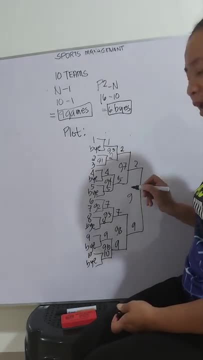 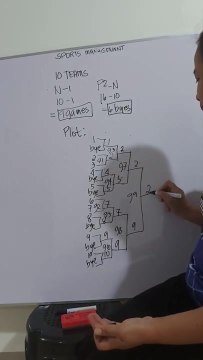 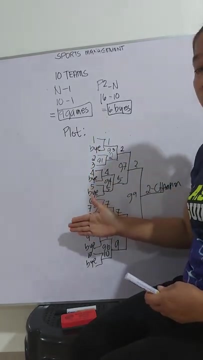 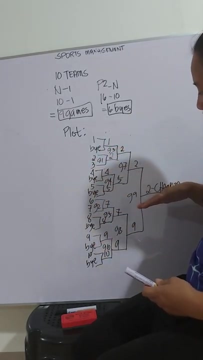 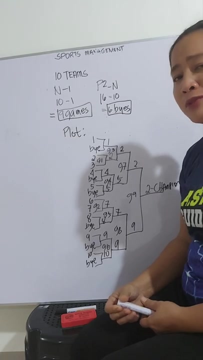 and team 9. this is our game 9. let's say team 2 is the winner. in other words, team 2 is the champion. in here you can write any number. you can have any of the teams here. example: you want team 9 as your champion, then it's up to you. but during final, then it's up to the players who can make it. 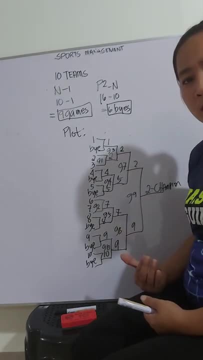 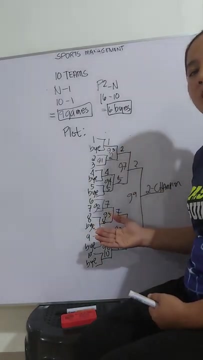 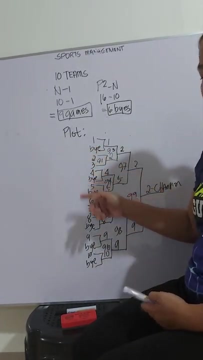 to the top of the game, and then it's up to the players who can make it to the top of the game or who can be the champion in the last round of the competition. i hope you learned something from the presentation, although you can make the other way. instead of having this kind of plot, you can.